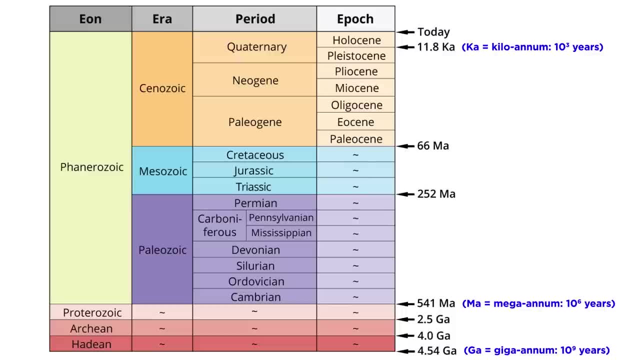 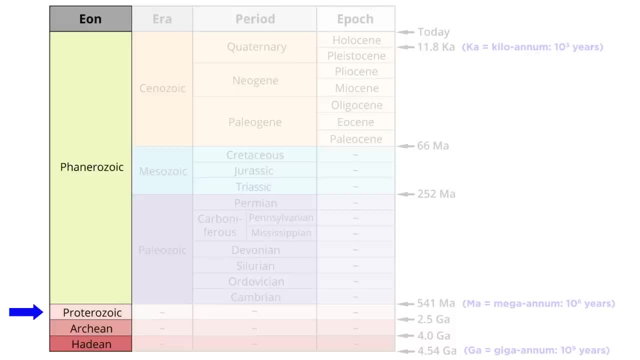 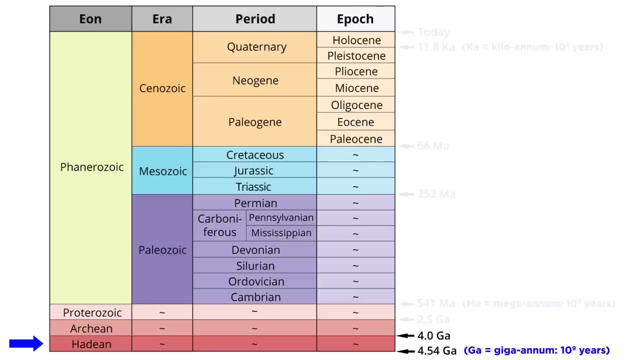 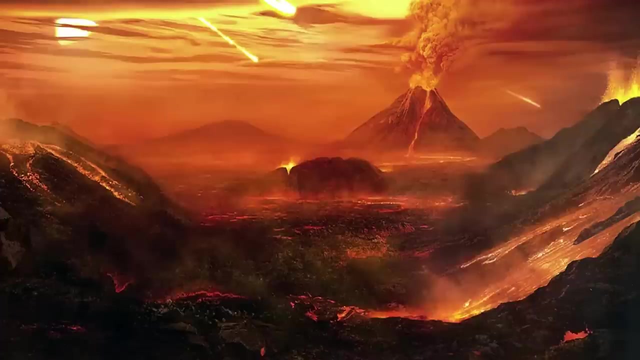 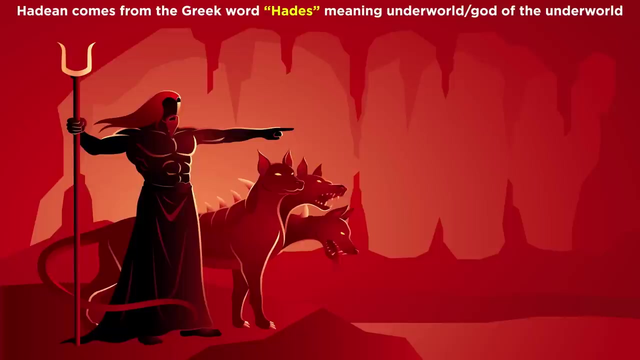 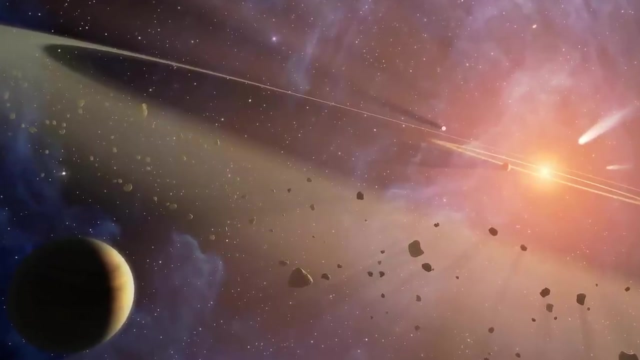 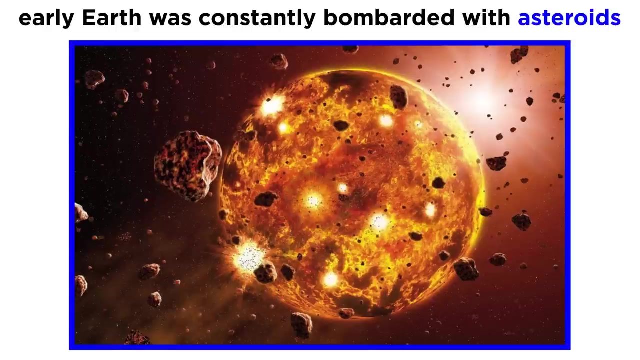 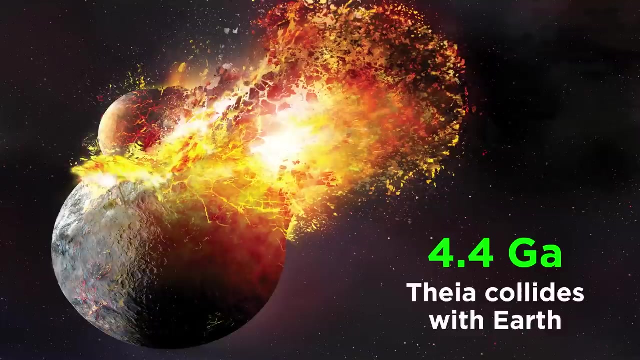 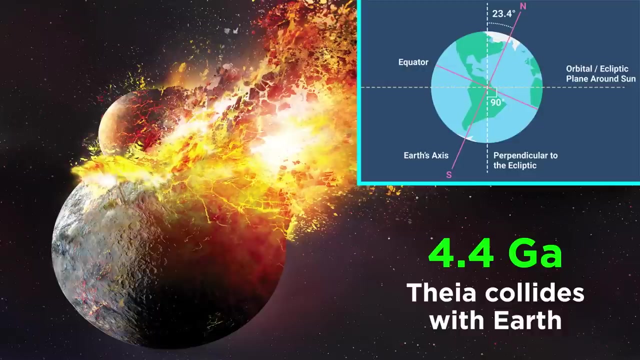 First, some terminology. In order to understand the timescales that Earth operates on, geologists came up with a way to break down the 4.57 billion years of Earth's existence. into smaller chunks called eons. There are four eons. These are the Hadean, Archean, Proterozoic, and Phanerozoic. In the earliest days of Earth's history, from 4.54 billion to about 4 billion years ago, Earth would have been unrecognizable to us. It was a hostile place with no continents, ubiquitous active volcanism, and frequent asteroid impacts. Given this description, it seems appropriate that this eon, the Hadean, is derived from the Greek word Hades, meaning the underworld, which is a fitting comparison to this hellish landscape. The frequent asteroid impacts were a result of the solar system being so very young, with huge numbers of large rocky bodies that had not yet been incorporated into planets or ejected from the system. A particularly notable event is believed to have occurred four point four billion years ago, when a Mars-sized protoplanet named Theia slammed into Earth, creating a worldwide magma ocean, and producing the tilt in Earth's rotational axis in the process. 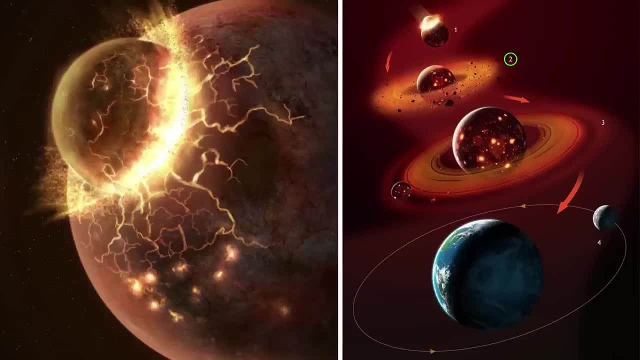 Though Earth and Theia mostly coalesced, the impact caused parts of the crust and mantle of both planets to be ejected into space, generating a ring of debris which collected to form our moon. 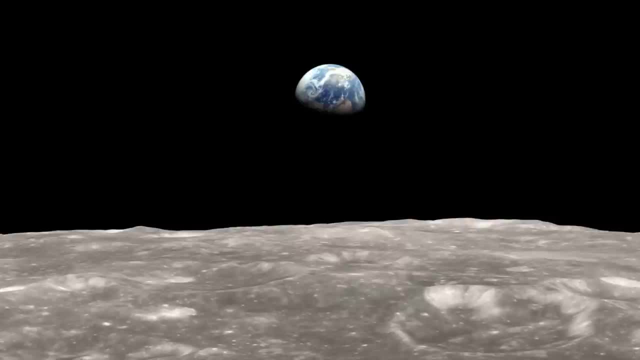 So interestingly, the moon is partly made of the Earth. After the collision, Earth began a slow journey toward more calm conditions, as protocontinents and oceans began to form. However, conditions were still extremely harsh 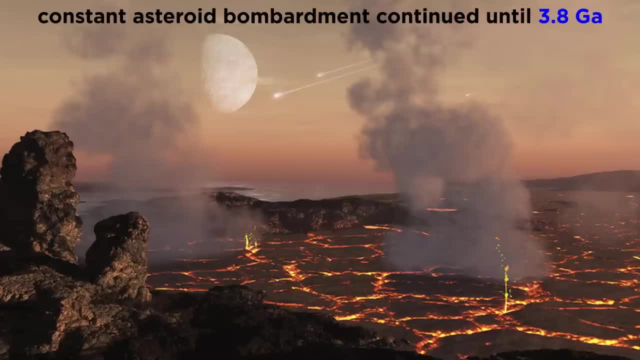 due to constant asteroid bombardment, which would continue until around 3.8 billion years ago. This likely hindered any development of life during this time. No rocks of Hadean age exist in the rock record, simply because older rocks are more likely to be 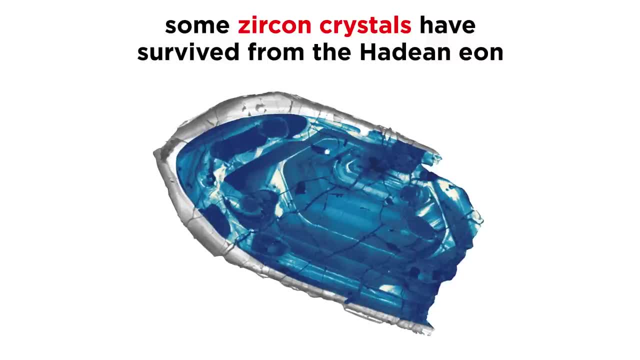 destroyed or altered by geologic processes. The only surviving terrestrial material from this time are zircon crystals, which are durable and can survive processes like subduction and weathering. 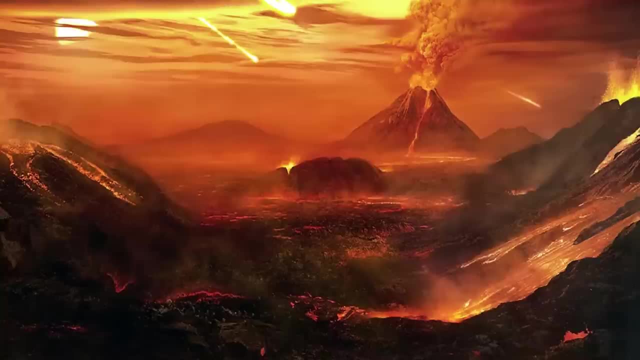 This makes the Hadean Eon the most mysterious time in Earth's history. 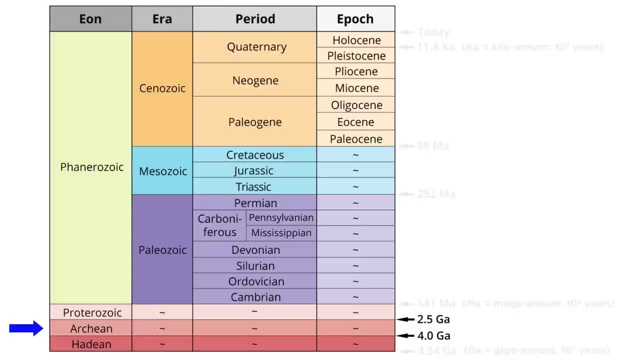 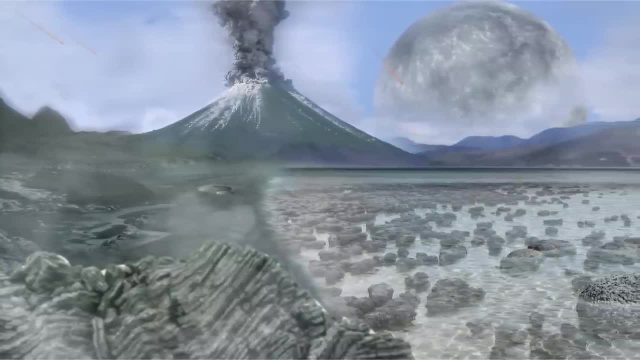 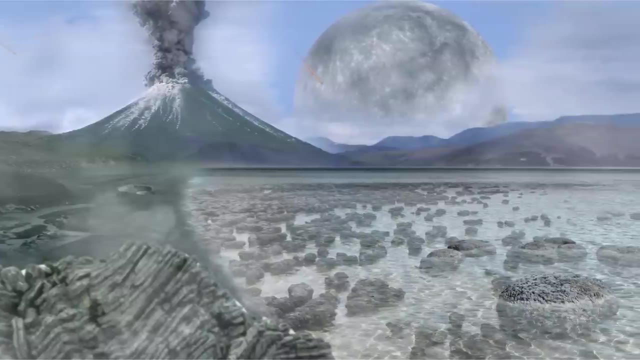 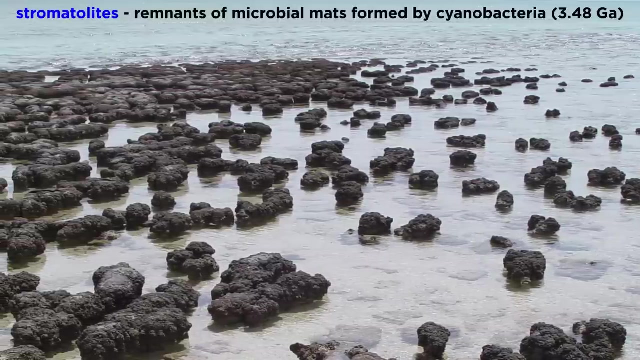 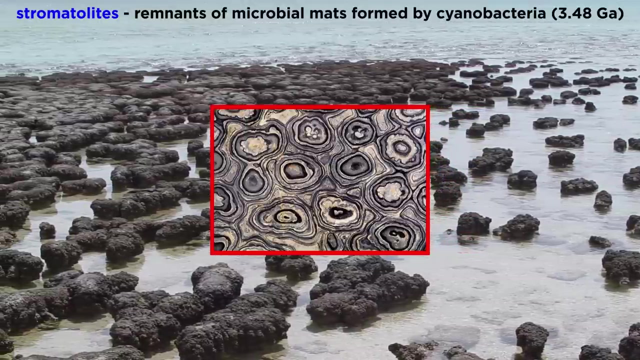 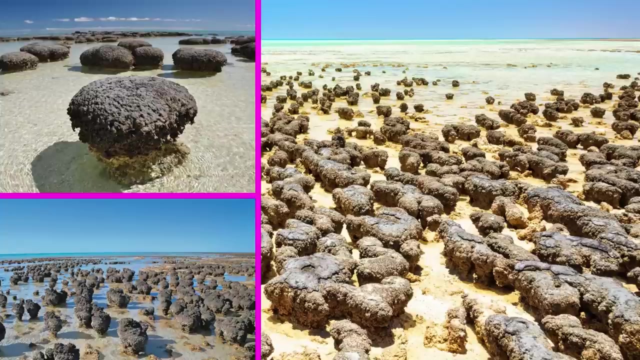 The next Eon, the Archean, lasted from four billion years to three billion years. This is a major billion to 2.5 billion years ago. One of the most important events in the Archean was the tapering off of heavy asteroid bombardment and the subsequent emergence of life. The oldest terrestrial rocks as well as fossils come from this eon. The oldest fossils are 3.48 billion year old stromatolites, which are the rocky remnants of microbial mats formed by cyanobacteria living in tidal flats. The abundance of these fossils suggests that by the Archean, single-celled life was already flourishing on Earth. 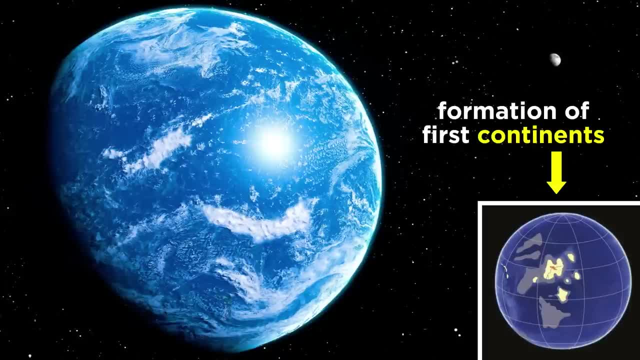 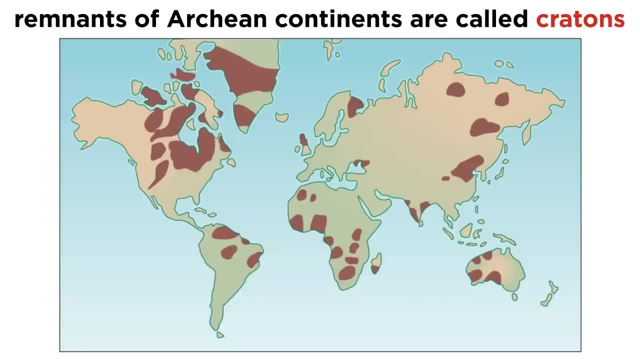 Another main event of the Archean was the formation of large continents. Remnants of these ancient continents are called cratons, and are found mainly in Canada, Africa, and Australia. 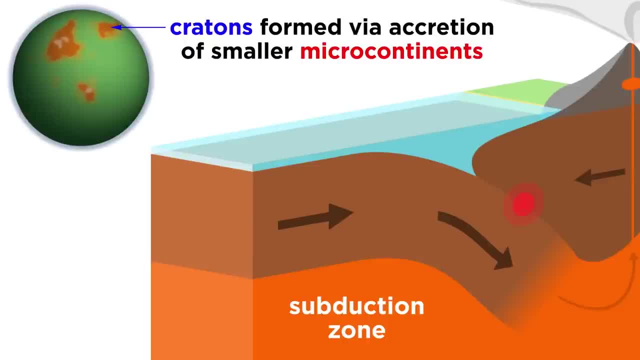 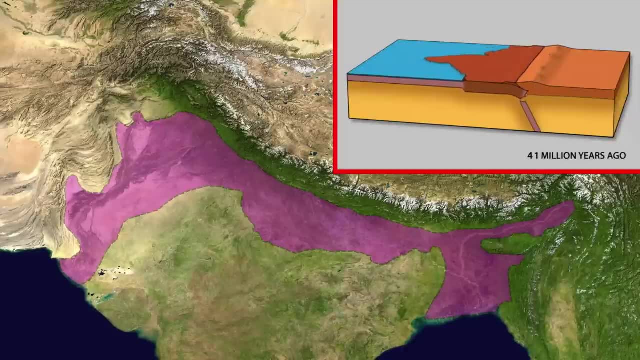 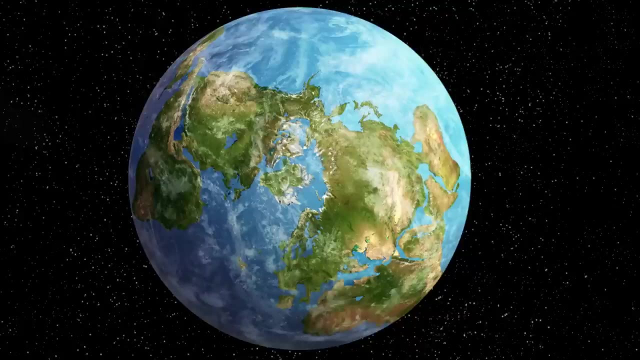 The cratons formed via accretion of the Archean. These cratons formed many smaller micro-continents as they collided along ancient subduction zones. This is essentially the same process that caused India to collide with Asia to form the Himalayas, just on a much larger scale, and which will eventually cause North America 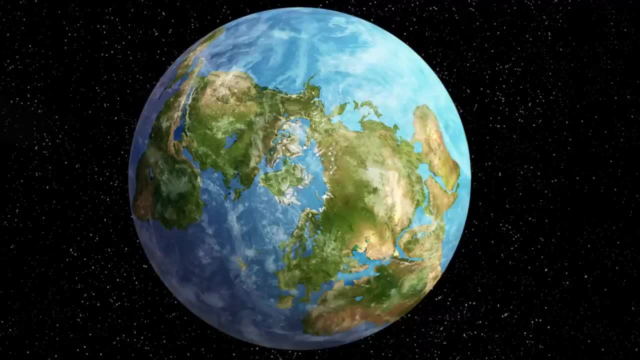 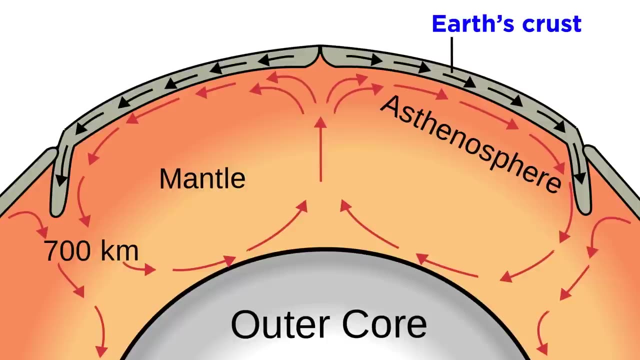 to collide with Asia hundreds of millions of years in the future. This is a good time to mention that Earth's crust, or outer layer, is broken into rigid chunks and pushed around by the conduction of these cratons. This is a good time to mention that Earth's crust, or outer layer, is broken into rigid chunks, and pushed around by the conduction of these cratons. 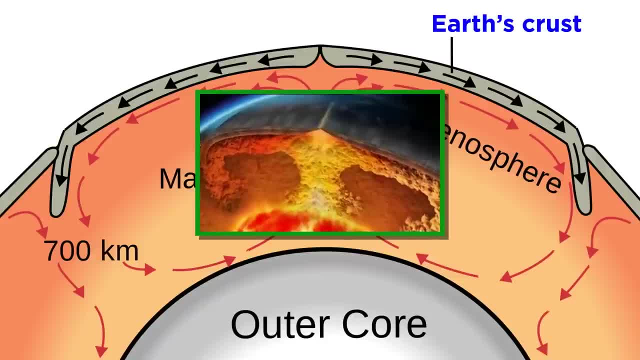 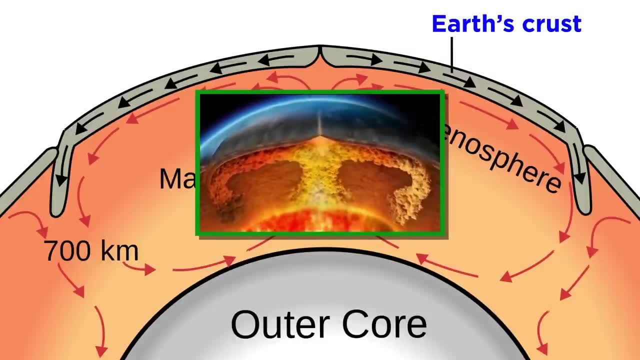 This is a good time to mention that Earth's crust, or outer layer, is broken into rigid chunks, and pushed around by the conduction of these cratons. 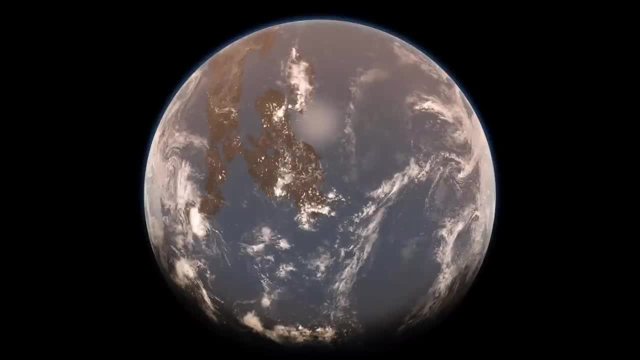 By the end of the Archean, Earth looked more or less like it does today, having oceans and large continents with rivers and lakes, but in other ways, it was still very different from the Earth we know. 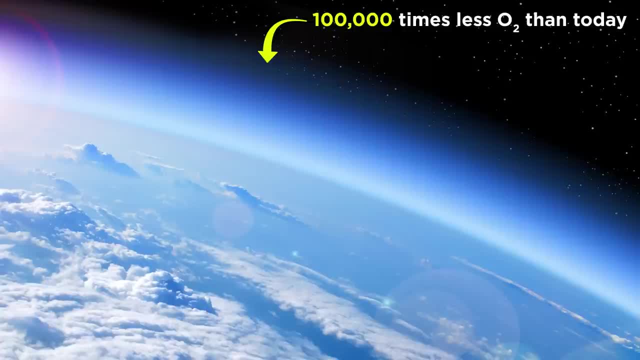 The Earth's atmosphere, for instance, had 100,000 times less oxygen than the air we're breathing right now, instead containing large amounts of carbon dioxide and methane. Life was also 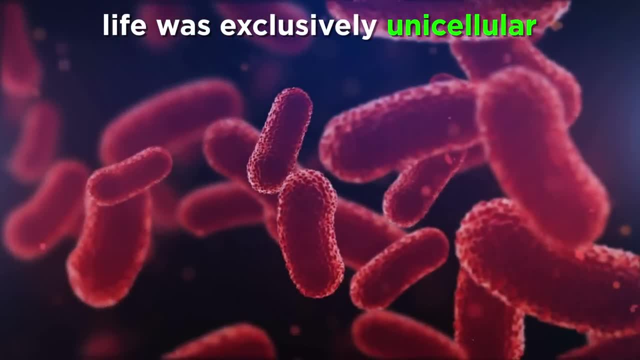 exclusively unicellular and would continue to be so for at least an additional billion years. 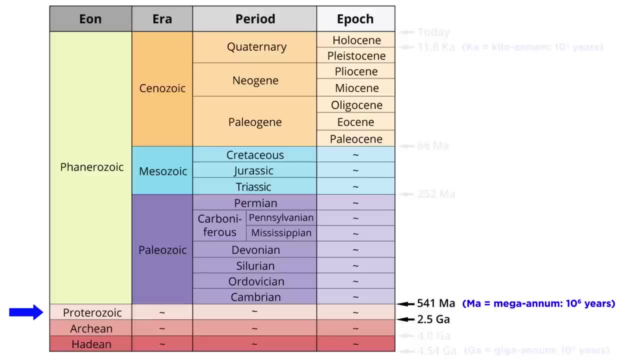 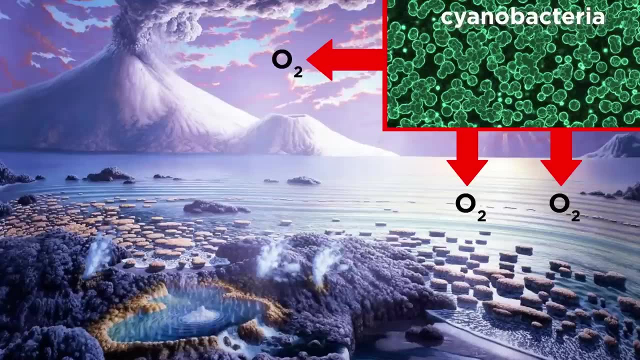 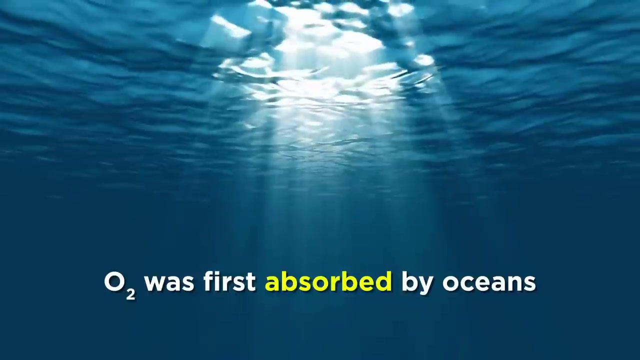 The next eon, the Proterozoic, lasted from 2.5 billion years ago to 541 million years ago, and began with a gradual increase in atmospheric oxygen, which was generated by newly evolved cyanobacteria with photosynthetic capabilities. This oxygen was absorbed by the oceans at first, which acted as a buffer preventing a rapid increase in atmospheric oxygen. 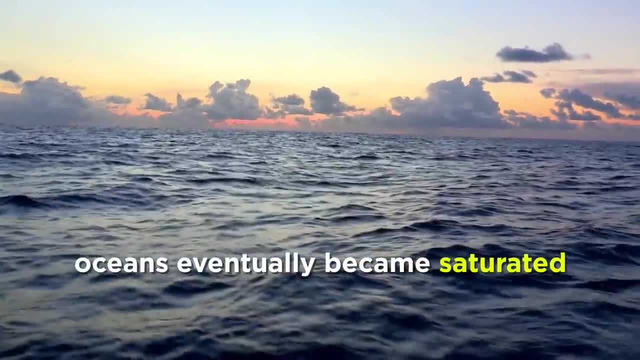 But the oceans eventually became saturated with oxygen, allowing atmospheric oxygen levels to rapidly soar, increasing by a factor of 100. Banded oxygen. Banded oxygen. 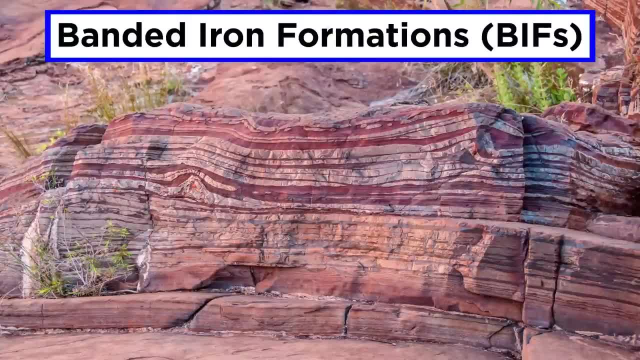 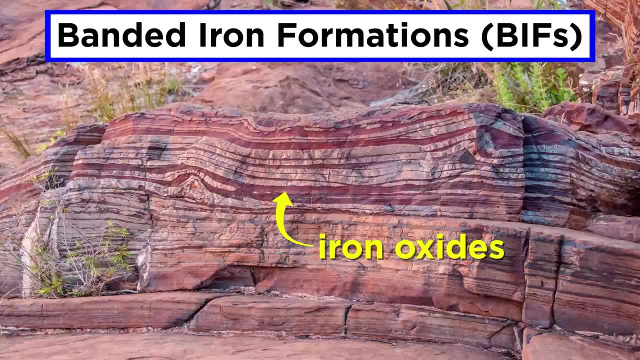 Iron formations, or BIFs, are marine deposits from this period and are characterized by thick deposits of iron oxides which precipitated from ocean water as oxygen concentrations increased. 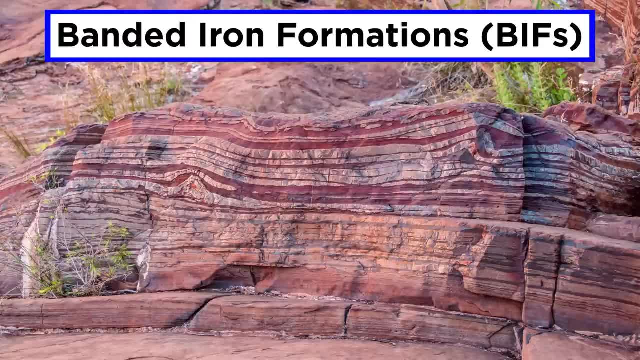 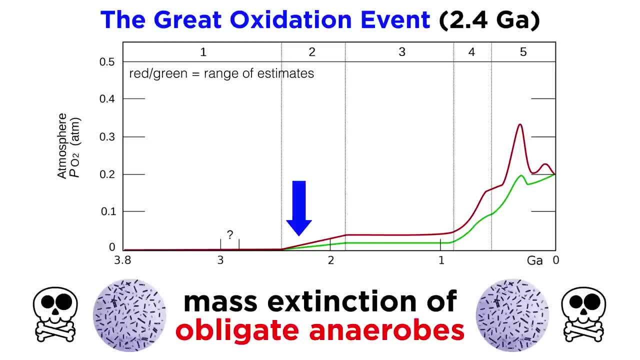 BIFs were not formed during any other period of Earth's history. The rapid increase in oxygen in both the atmosphere and oceans caused a mass extinction of obligate anaerobes, which are organisms that are poisoned by oxygen. This event is called the Great Oxidation Event, or perhaps from the perspective of the 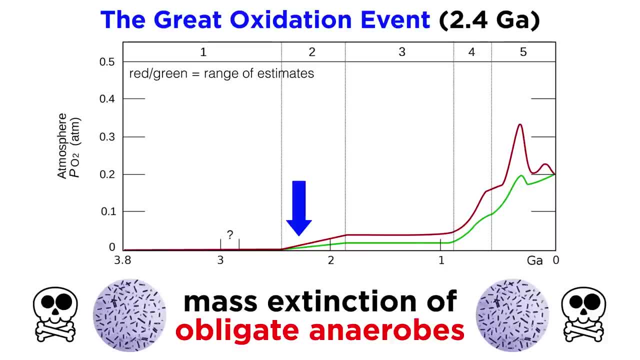 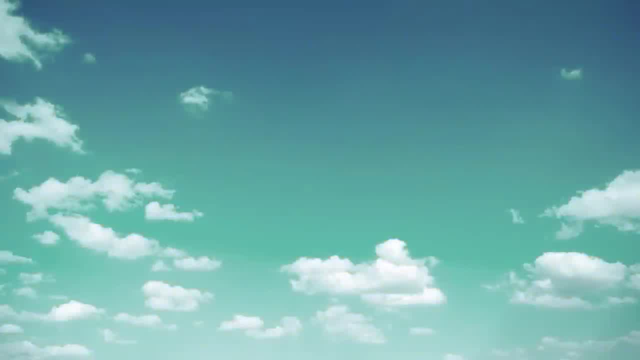 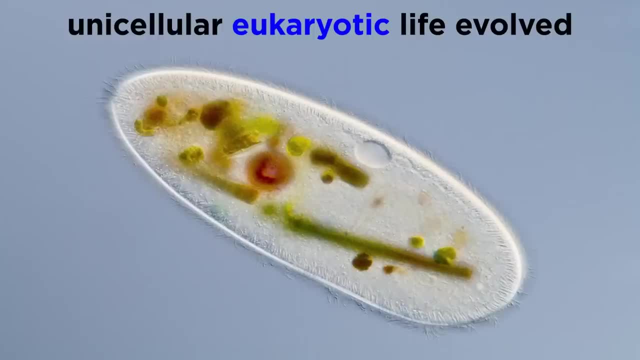 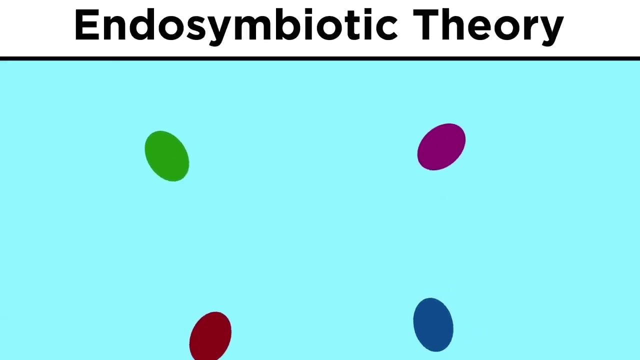 anaerobic organisms that abruptly died, the Great Oxygen Catastrophe. Additionally, the skies and oceans shifted from orange and green-tinted to the blue we see today. The evolution of unicellular eukaryotes occurred during the Proterozoic. As we learned in the biology series, these are single-cell organisms containing nuclei and other highly specialized organelles, like mitochondria and chloroplasts, through a process called endosymbiosis, where certain prokaryotic organisms 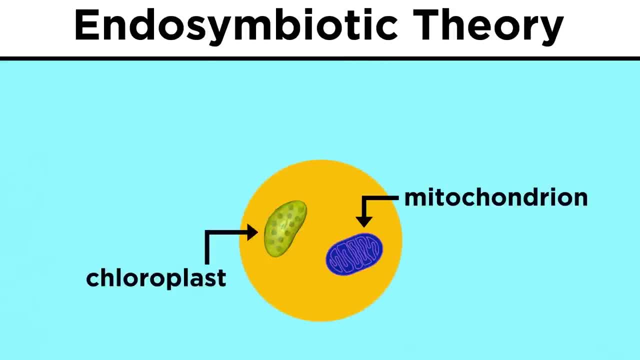 were incorporated into others, with organelles like mitochondria and chloroplasts being derived from the eaten prokaryotes, so to speak. 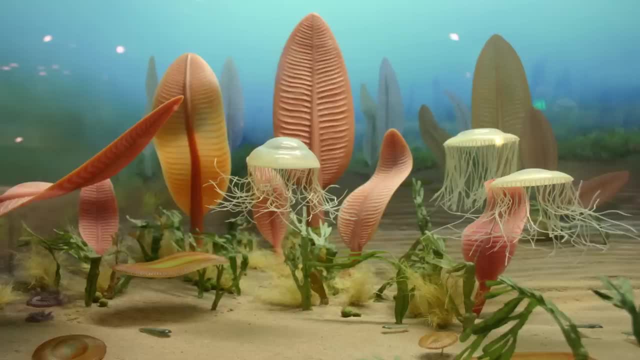 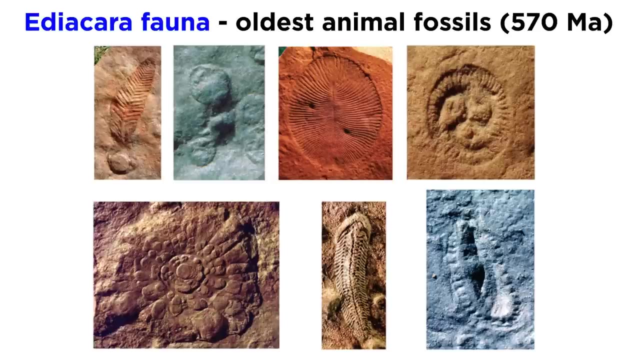 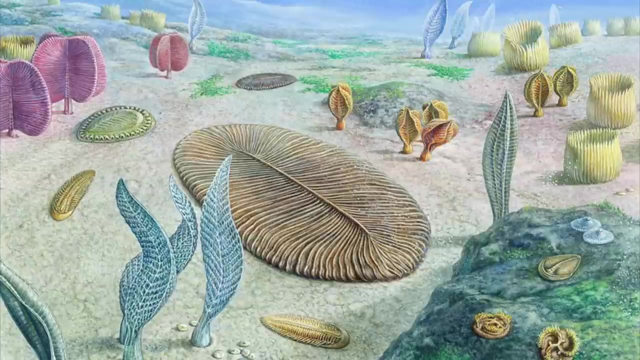 The first multicellular life, and even animals, also evolved during the Proterozoic. The oldest indisputable animal fossils are from 570 million years ago, and are called the Ediacara fauna. Some examples of these primordial fauna are Charnia, a frond-like animal, Sprigina, a worm-like animal, and Chimborella, a mollusk-like animal. The large diversity of animal 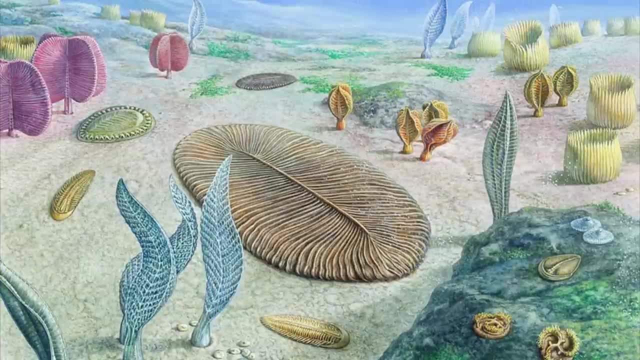 fossils present in these rocks indicates that animals were rapidly evolving as nature experimented with different body types. 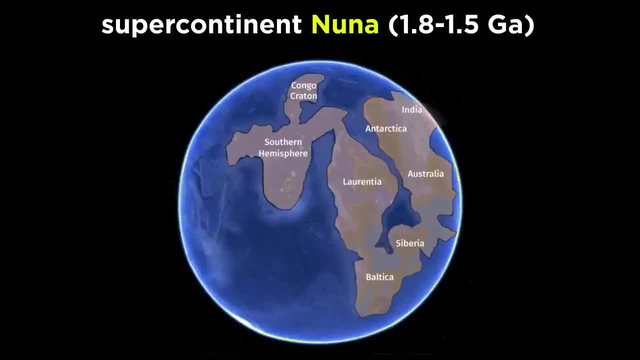 The Proterozoic was also a time of supercontinents. Converging continents collided around 1.8 billion years ago to form the first supercontinent, called Nuna. However, around 1.5 billion years ago, convection currents in the mantle changed direction, causing Nuna to break apart, or rift. 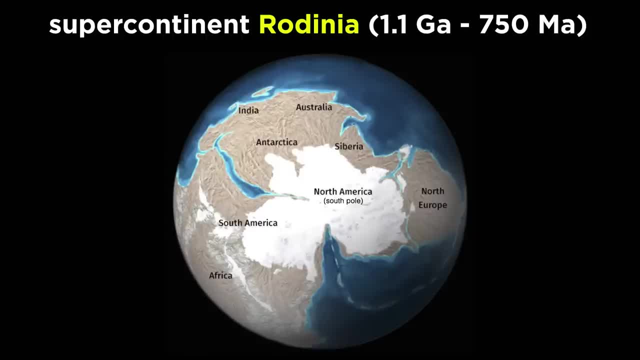 The assembly and later breakup of supercontinents is a cycle that was to repeat an additional two times in Earth's history, with another cycle occurring later in the Proterozoic with the formation and breakup of Rodinia between 1.1 billion and 750 million years ago. 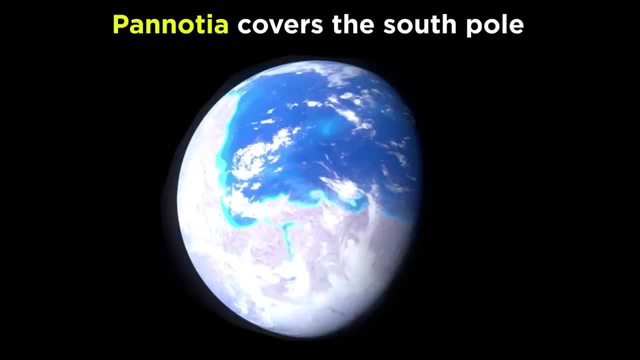 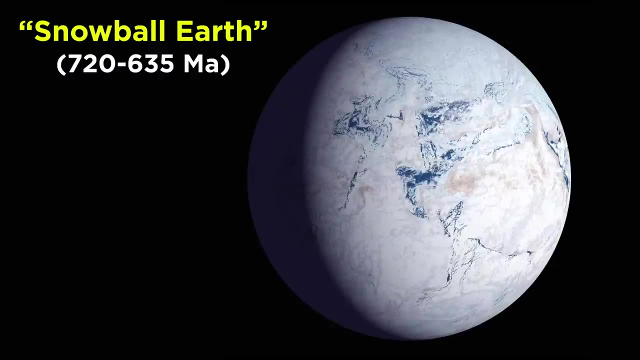 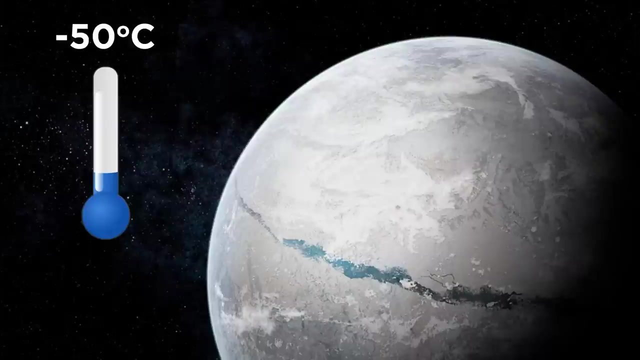